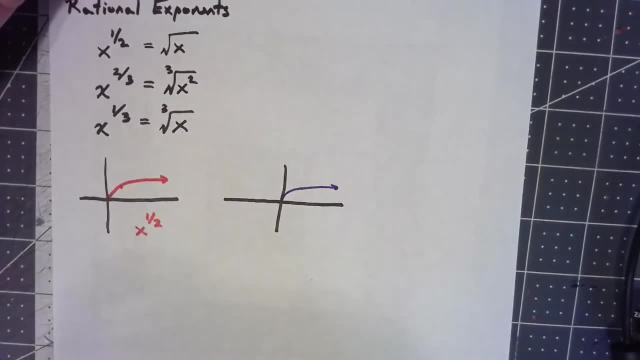 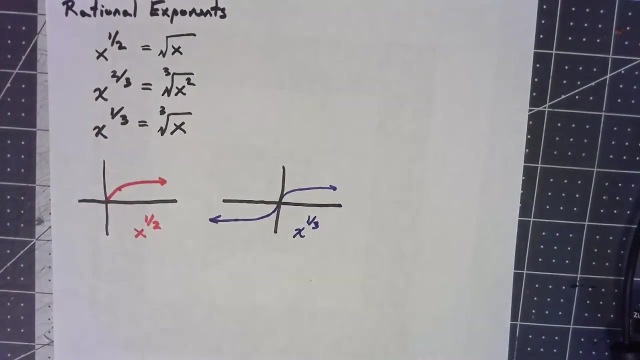 out a little bit more, but, honestly, you probably wouldn't notice that if you were just looking at a graph. But the big thing is is that it also is an odd function and does the same thing over for the negative side. Now, the thing about those two graphs, just like when 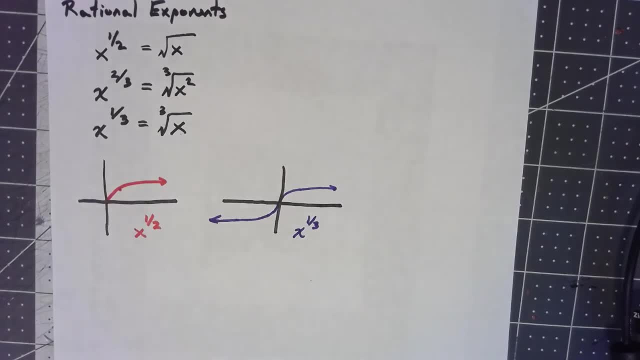 we talked about. the graph of x squared was very similar to the graph of x to the 4th, x to the 6th, x to the 8th, any positive Even power. It's a similar kind of thing. here. These graphs look very similar to a bunch. 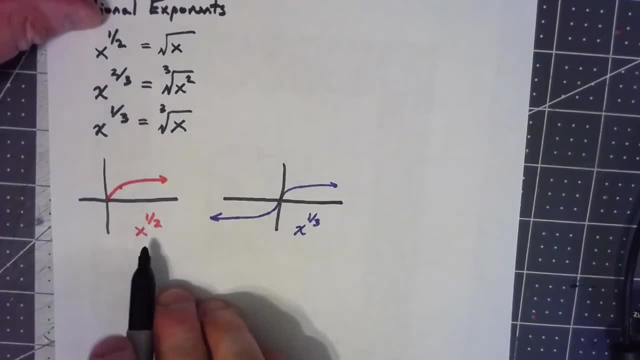 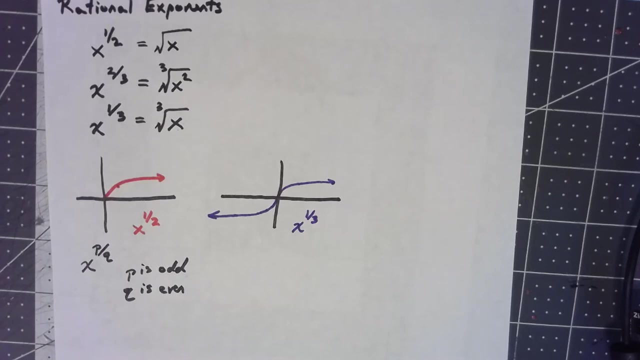 of others, In particular this one here. any time when you've got x to a power, that's a fraction and p is odd And Q is even. Any time the top of the fraction is odd and the bottom of the fraction is even. 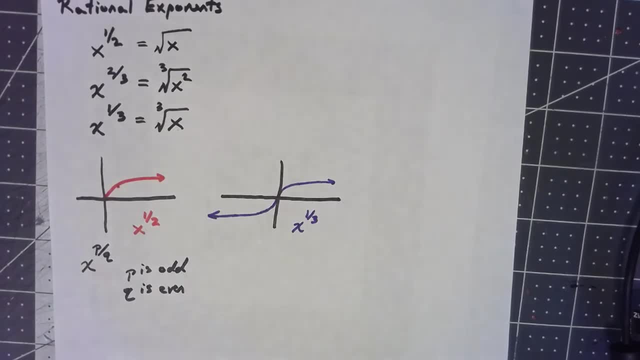 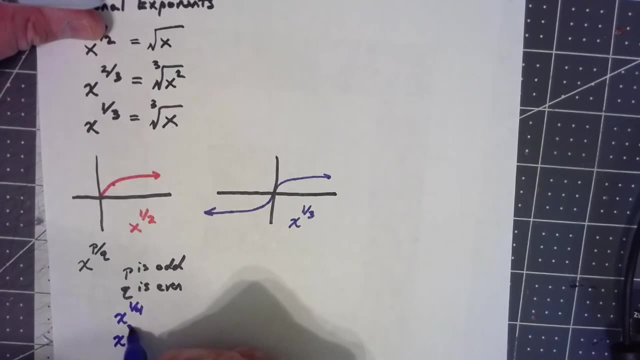 it's going to look like this, So just throwing out a few. so x to the 1, 4th is pretty much going to look like that. X to the 3, 8ths is going to look like that. X to the. 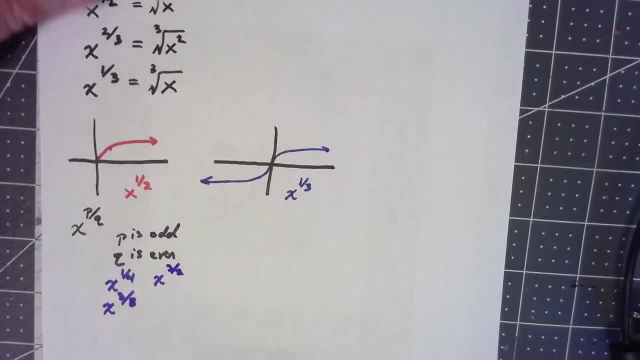 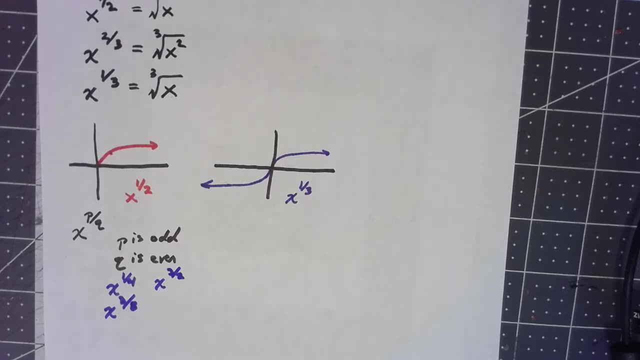 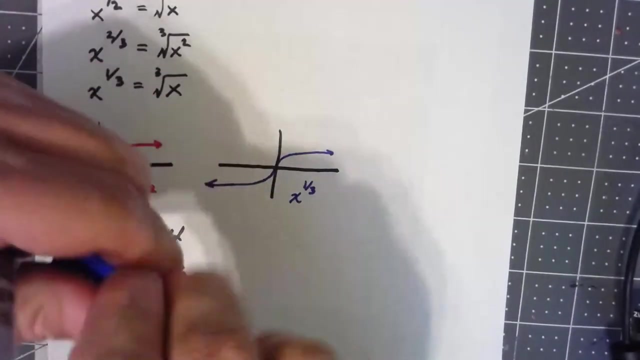 Up, Up, three halves is going to look like that. anytime, the top of the fraction is odd and the bottom's even actually let's. let me change that a little bit. I'm going to throw it x to the three halves out, let's. and because there is another rule here, that the bottom has to be bigger than the top. 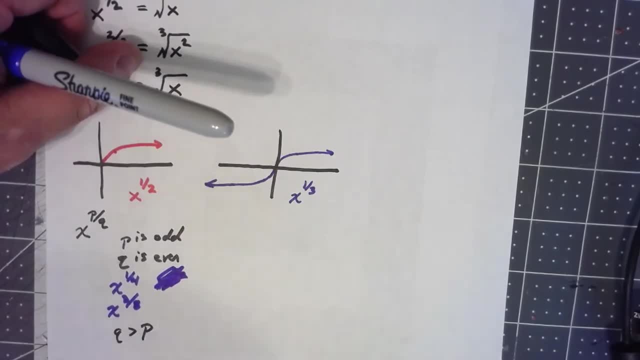 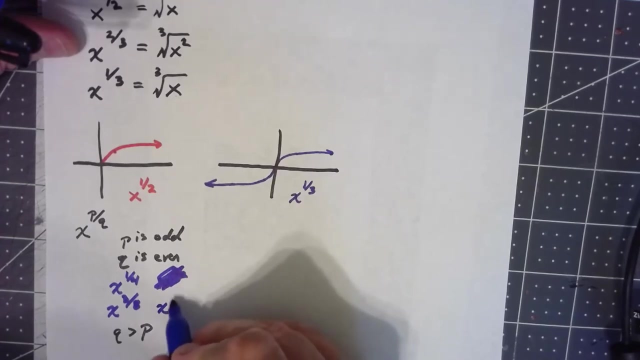 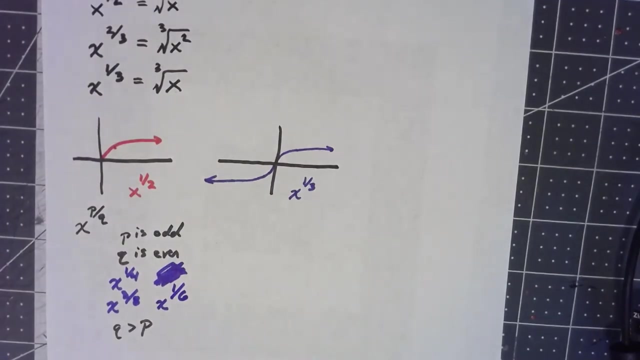 we're only looking at actual things that are less than one. we're looking at these graphs, so, but at the same time, something like X to the oh, one sixth would look like this: this one here, it's the same kind of thing. anytime I've got something where I've got X to a fraction and 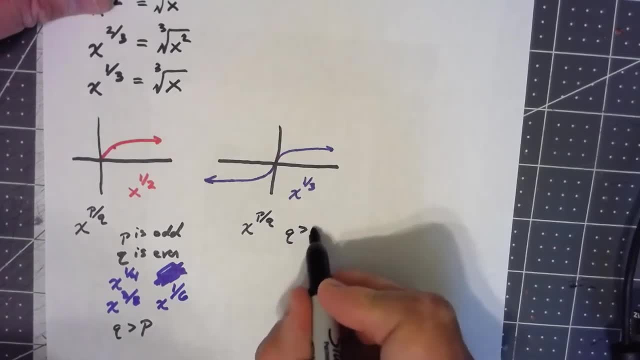 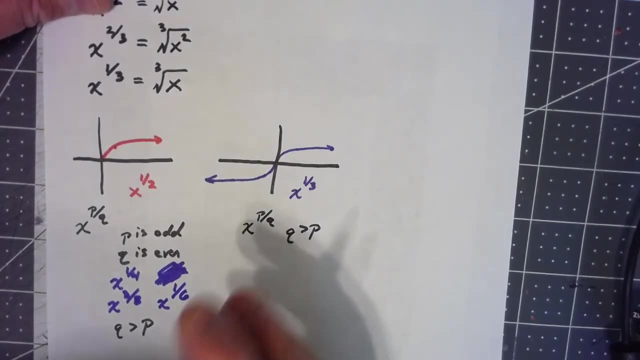 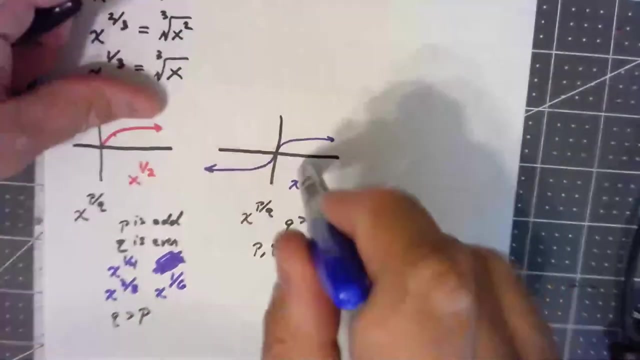 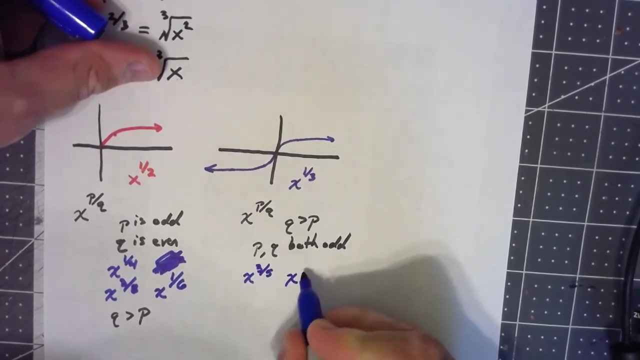 the bottom is bigger than the top, and this one is that both the top and the bottom are odd you so the same basic shape here would apply to X to the 3 fifths, X to the 1 seventh, X to the 5 ninths. anytime, both the top and the bottom are odd numbers and again the bottom has to be bigger. 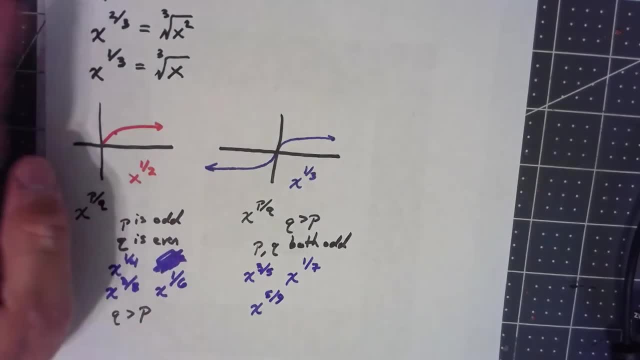 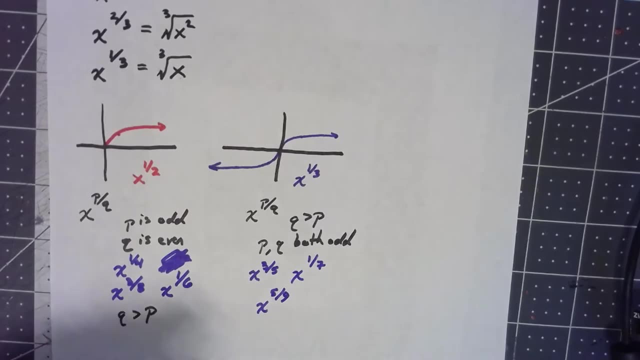 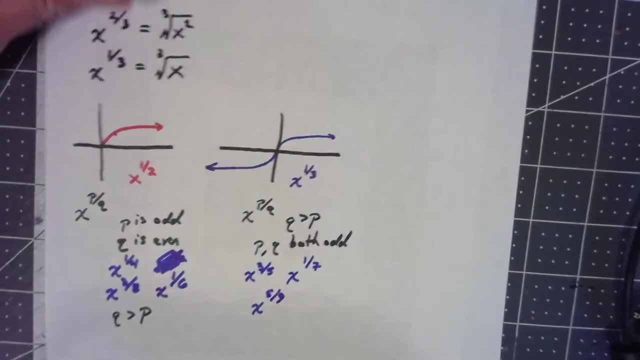 than the top. but what about this X to the 2 thirds? notice that both of these things had the top number being odd and the bottom has to be bigger than the top. but what about this X to the 2 thirds odd? And this x to the 2 thirds has the top number being even. Well, this one. 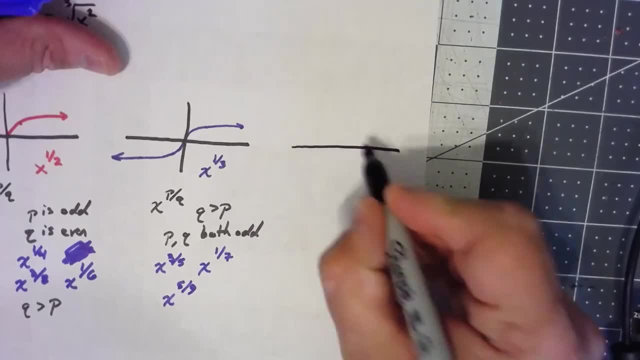 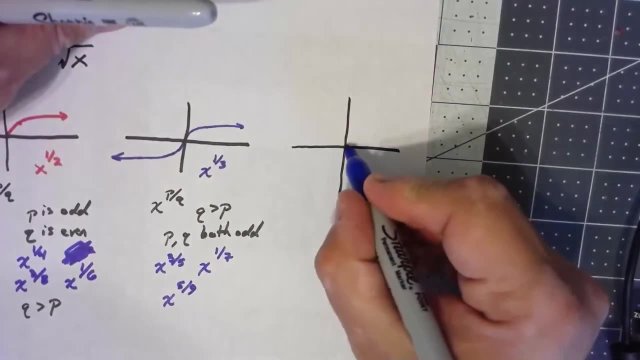 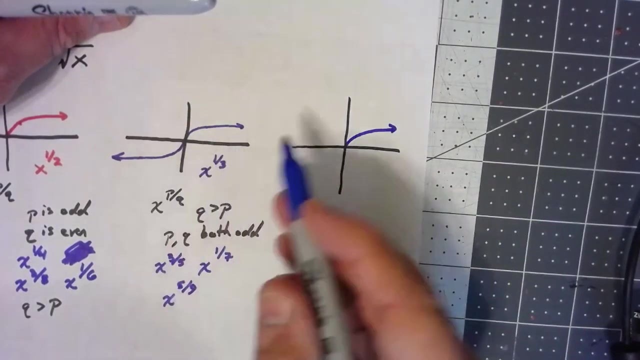 looks just a little bit weird. It still has the same basic shape over to the right that both of the others did, but instead of going down like this and being an odd function, it's actually an even function. It's symmetric about the y. 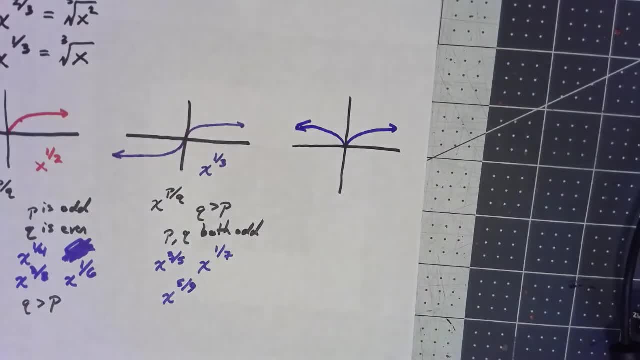 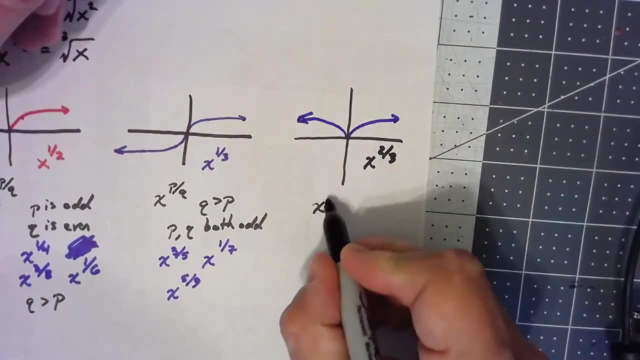 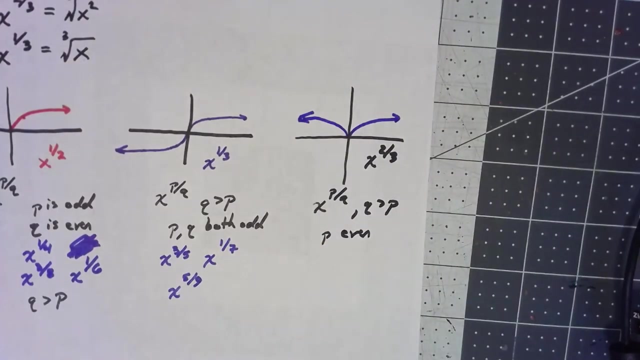 axis. Now again, this is x to a fraction. The bottom has to be bigger than the top. In this case, the only thing that matters is that the top is even. It doesn't matter whether we've got an even or an odd number on the bottom, as long as the 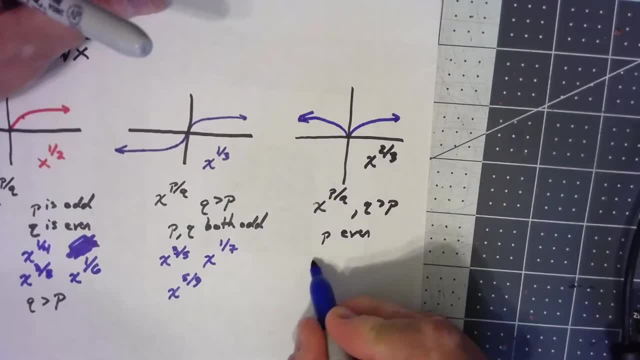 top is even. So I said, if we got x to the 2 thirds, if I had x to the 2 fifths, if I had x to the 4 sevenths, if I had x to the 2 sixths. Now just one last thing and 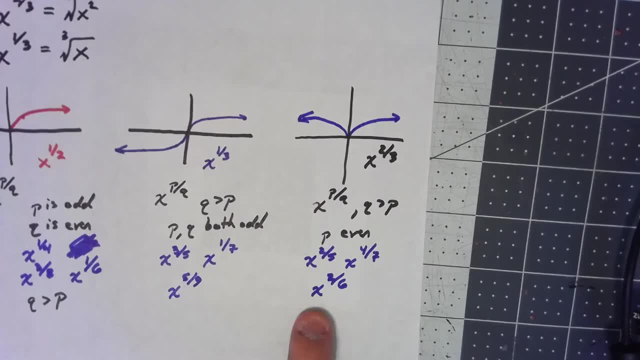 this is something that's really subtle here. Notice that x to the 2 sixths is different from x to the 1 third. This one has a graph that looks like this: This one has a graph that looks like this: Now,